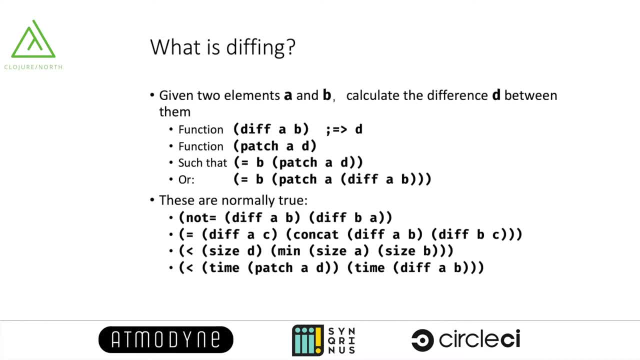 also addictive. concatenating the diff of A and B with the diff of B and C, you will get back diff of A and C. These two properties make diffing an ideal tool for tracking changes. Moreover, the size of the differences- D- is normally much. 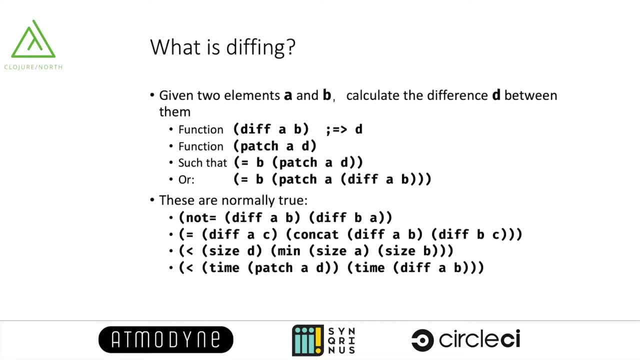 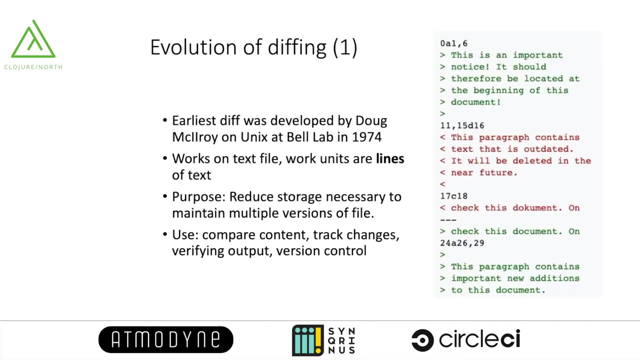 smaller than either of the original A or B, making it suitable for data storage and data transmission over networks. Finally, it is much quicker to run patch than to run diff, so data recovery from diffs is normally quick and cheap. So not surprisingly, as early as 1974,. 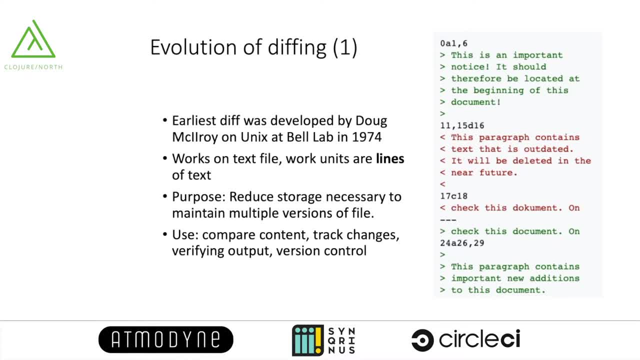 the diff of D is much smaller than D of E. This is not a big deal. This result is: Diff and Patch have been developed as Unix programs by BearLab. These programs have been widely used even to today. These programs work with line of text and are mainly useful for comparing text files. 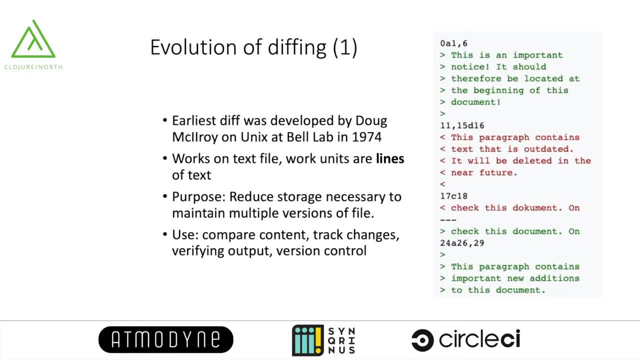 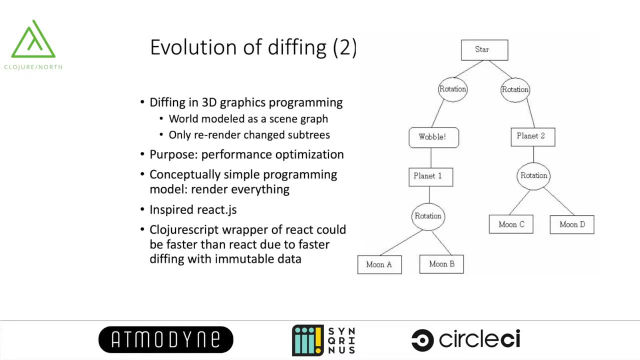 tracking changes, verifying output or being used in version control systems. Since 1980s, additional use of Diffing happened in the 3D computer graphics community. In the scene graph approach of computer graphics rendering, the world is modeled as a scene. 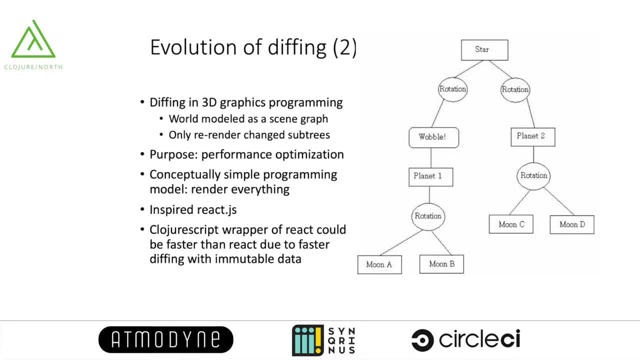 graph. The rendering engine traverses the graph to render the scene under strict time requirements. For example, it must finish rendering a frame within 30 milliseconds. So in order to meet the frame requirement, it must finish rendering a frame within 30. 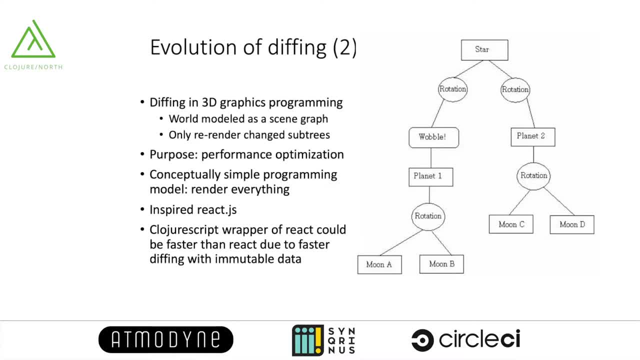 milliseconds. To meet those requirements, one of the performance optimizations used is to only render the changed subtrees in the scene graph, So this requires diffing the scene graph of the current frame with that of the previous frame. The benefit of this rendering approach is that it has a conceptually simple programming. 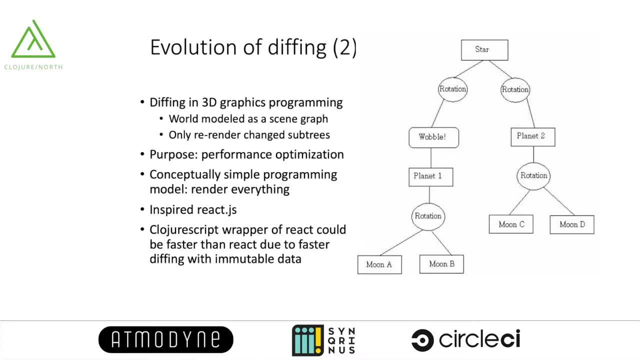 model Programmers can pretend that everything is re-rendered in every frame. This is a very useful feature, Thank you. So this conceptual simplicity inspired the popular React web rendering framework, where a career script wrapper of React could actually be faster than React itself sometimes. 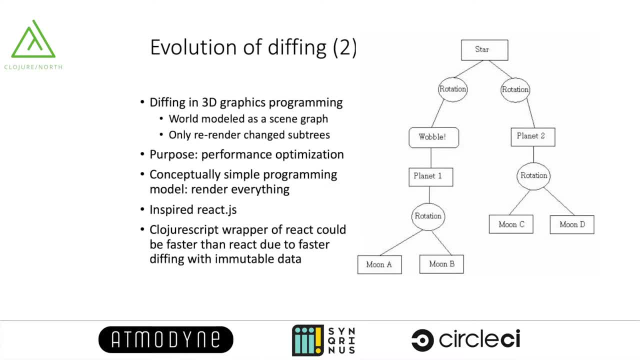 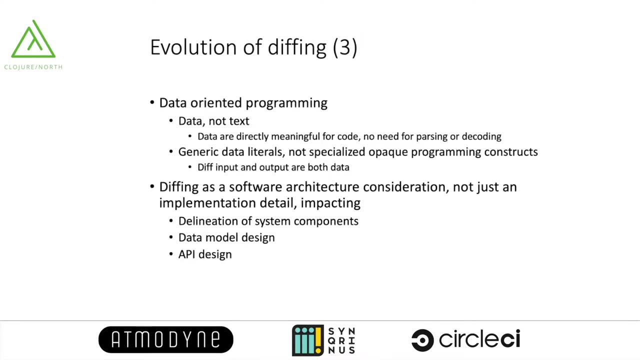 Due to these career scripts, immutable data structure enables faster rendering by producing faster diffing. So in Clojure we would like to work with data. So we are not going to be diffing text, instead we will be diffing data. Also, we would like to run diffing on generic data structures, not specialized programming. 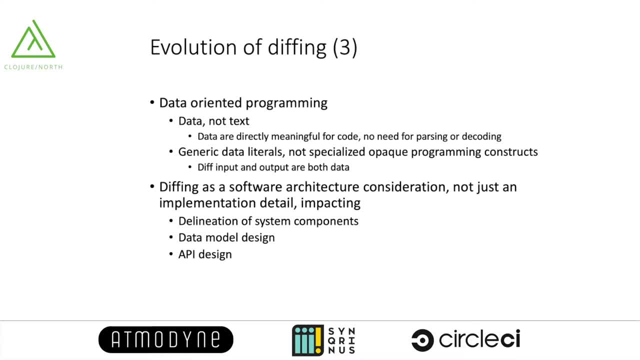 constructs wrapped in classes. So by taking advantage of generic, immutable data structures, we could elevate the data structure. This is a very useful feature, Thank you, Thank you. Next I will demonstrate the Data Diffing approach to the level of software architecture. 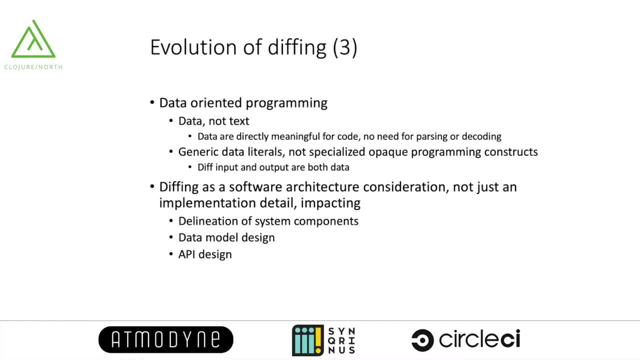 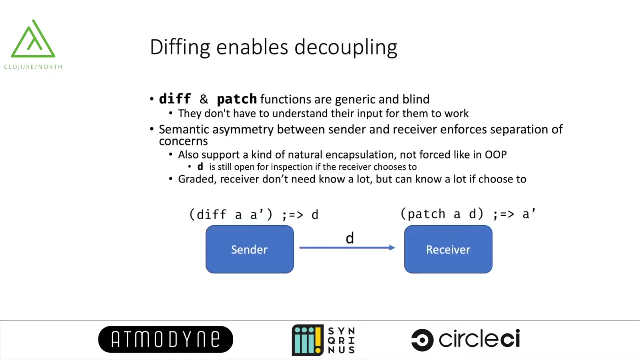 consideration, not just as an implementation technique useful only for performance optimization or data savings. Next, I will show that the use of diffing can have positive impact on system design, data modeling and API design. So the first benefit of diffing for software architecture stems from the generic nature. 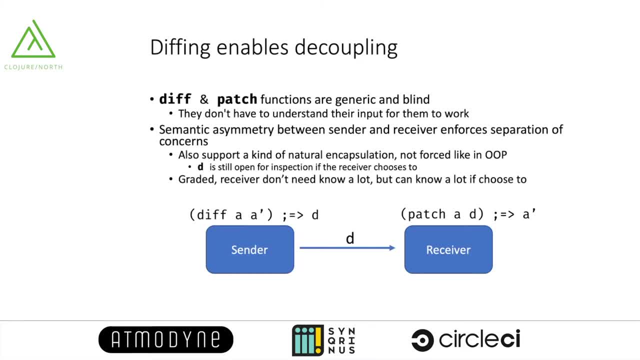 of diff and patch functions. In a sense, chief and patch are blend functions, for they don't have to understand the semantics of the input to do what they are designed to do. In the case of information sender and receiver, suppose the sender did some changes on its 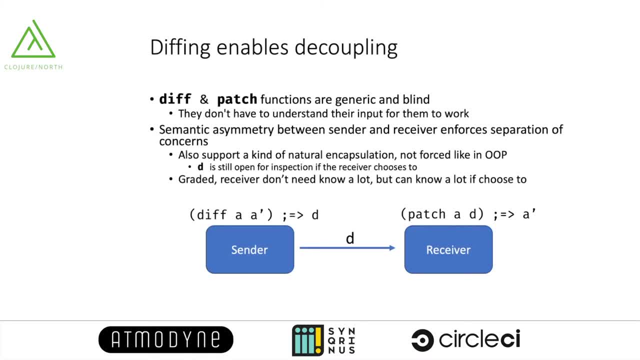 own data A to arrive at new data A'. it then computes the differences of A and A' and sends the diff to the receiver. The receiver does not have to know what the sender did with A. The process of turning A to A' may be quite involved, having lots of complexities. 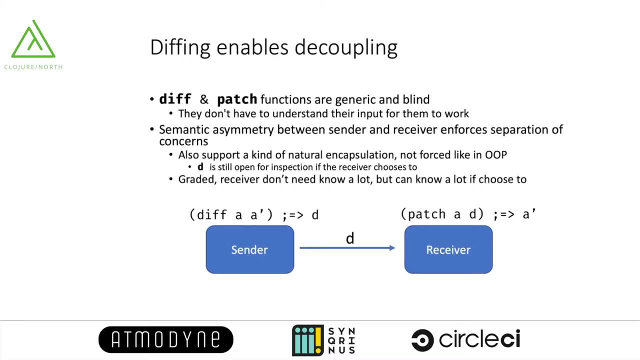 The receiver is oblivious to all of that. All it needs to do is to run patch on its copy of A with the received diff. It then gets the desired results A' without understanding much of what actually happened on the sender's side, Because the semantics of the changes on the sender's side can be completely opaque. for 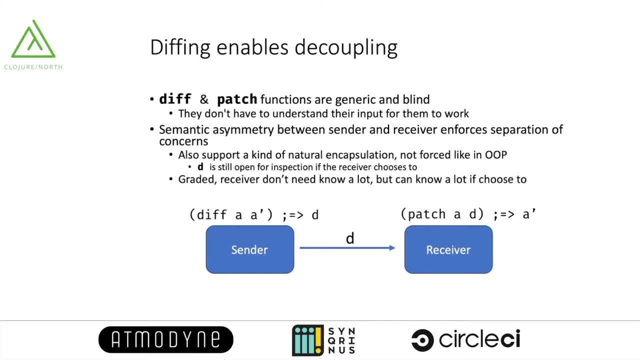 the receiver. this semantic isometry enforces the kind of separation of consents. It is also a kind of lateral encapsulation, but not forced like in object-oriented programming, Because the difference is D is still open for inspection. So this is a kind of graded decoupling. 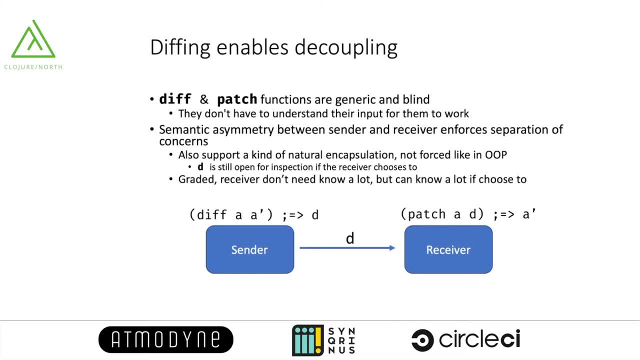 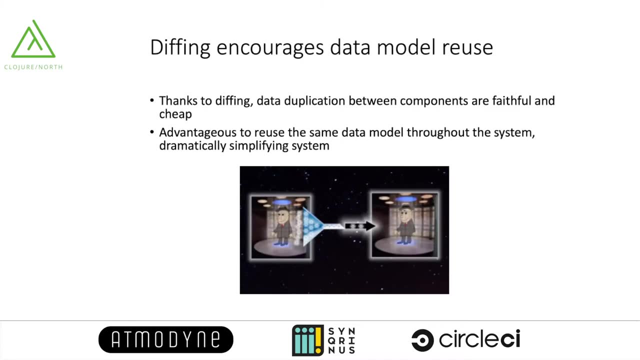 The data receiver don't need to know a lot for things to work, but it can also know a lot if it decided to inspect and record. Another architectural benefit is that diffing encourages data model reuse. A pair of diff and patch functions is like a pair of teleportation devices. 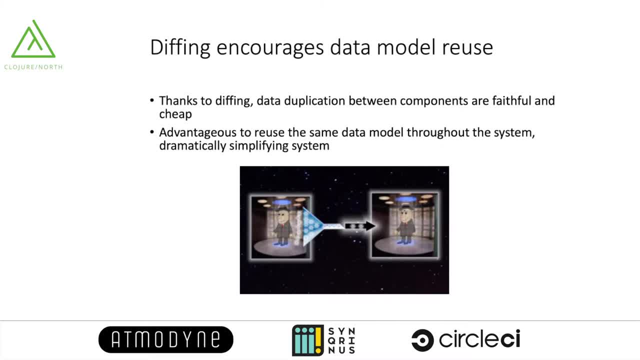 Data can be replicated on the other side without much fuss. Because data replication becomes cheap, it becomes beneficial to reuse the same data to the next generation. So this is a kind of graded decoupling same data model in different parts of the system, rather than each parts come. 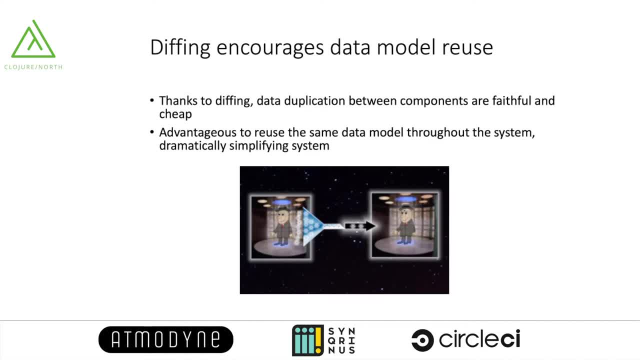 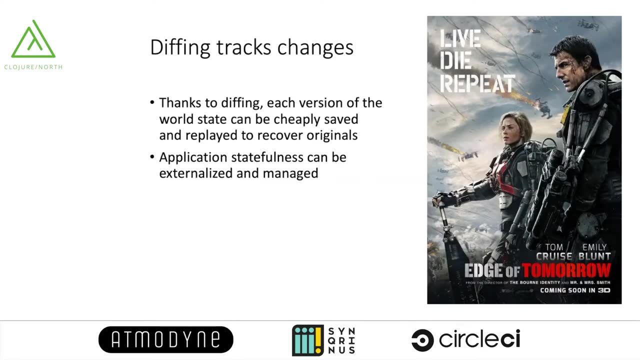 up with its own data models. This will dramatically simplify system design. As we know, most of our programming is just data transformation from one shape to another. Data model reuse saves a lot of work. Finally, Dfin is very good for tracking changes When each versions of the data 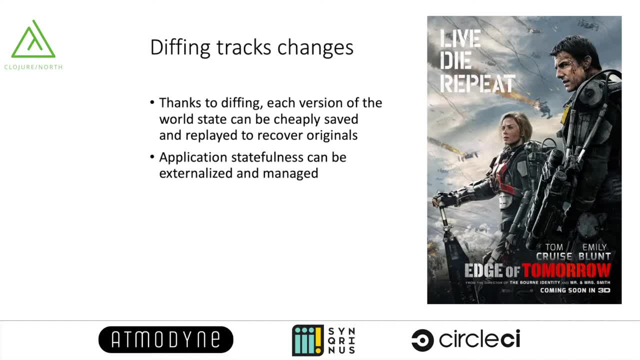 model can be cheaply saved and replayed to recover the original versions. a lot of interesting things can be done. For example, we can tweak the versions of the world to find one that suits our purpose, like in Tom Cruise's Age of Tomorrow movie. 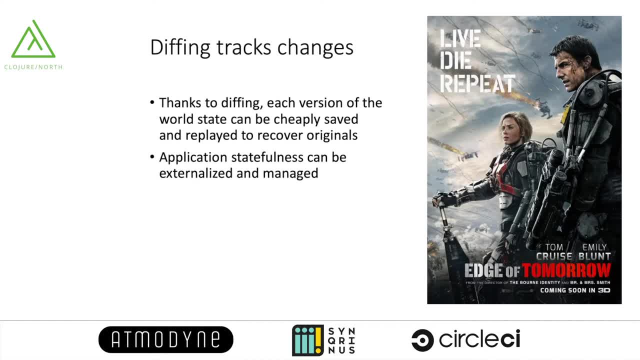 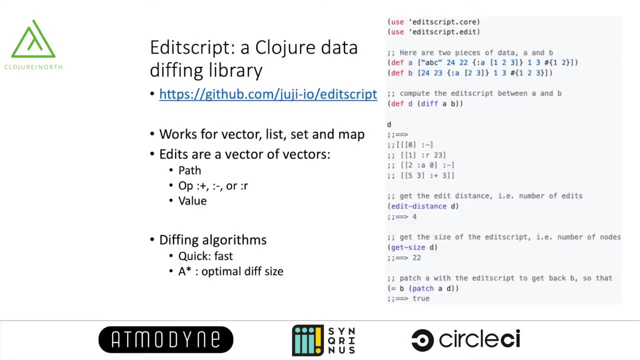 Cheap versioning also provides a way to manage the state of stateful applications, allow states to be externalized, achieving effective stateless architecture With stateful data models. In order to do all that, we have developed a data Dfin library for Clojure and ClojureScript. We call it EditScript- EditScript. 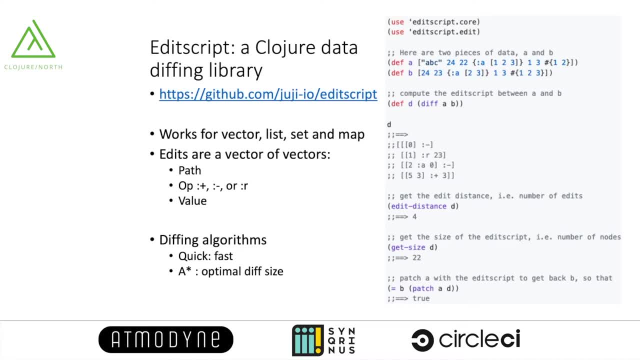 works on all regular Clojure data structures: vectors, lists, sets and maps. You can also implement our protocols to handle your own custom data structures. The Dfin library offers a wide range of options for monitoring any data model that we want to date and compare to the current ones. 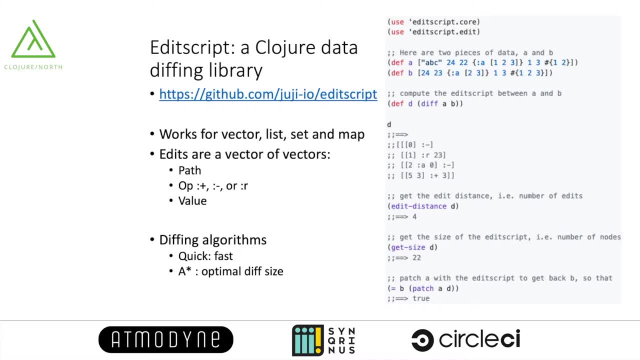 produces by edit script is a vector of edit. each edit is a vector of three or two elements: the path, the operator, which include add, delete and replace, and finally is a value for add and replace operation. two different algorithms are provided in edit script. a quick algorithm is very fast but it produces 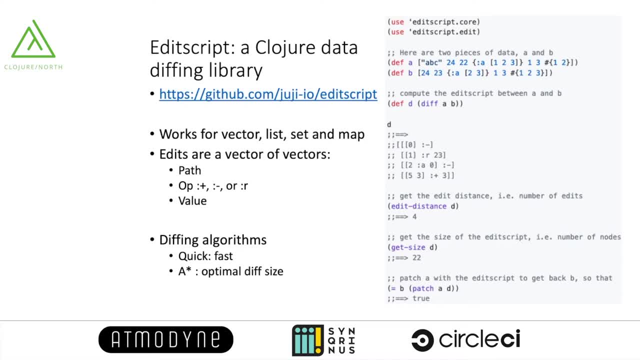 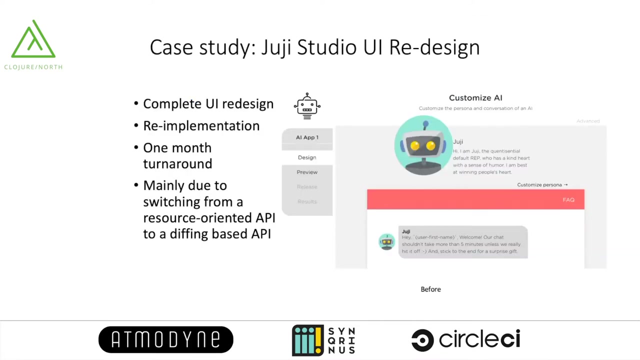 sub optimal diffing in terms of size, and another, a star algorithm, which is slower but produce optimal diffing in size, depending on your use case. both algorithms are quite useful in practice. we have been using edit script in production for a couple of years, so we one major use of edit script that saved us a lot of time and efforts is in our 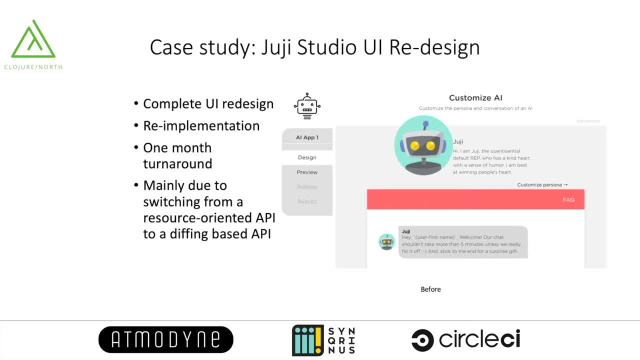 recent user interface rewrite for our 2g studio product. 2g studio is a GUI tool for users to create AI driven chatbots. as the product grows in features, we started to feel that changes become harder to make and UI iterations become slowed down, compounded with some usability issues. we decided to rewrite the user interface. 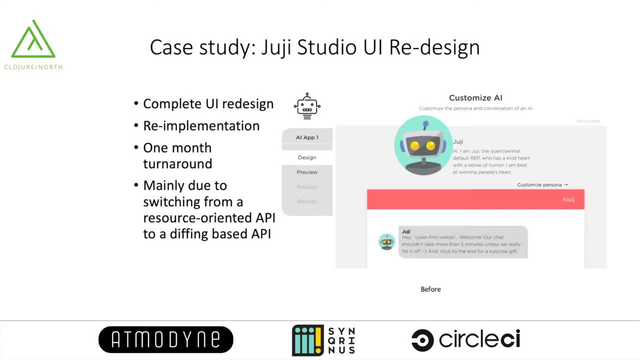 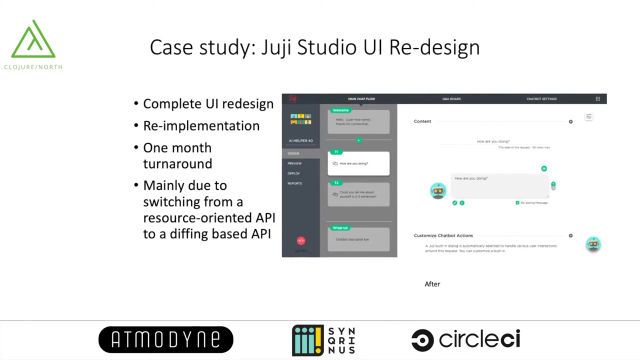 this rewrite turned out to be a major success. it was done very quickly, within a matter of months. the rewrite included both UI redesign and re-implementation, so this is a screenshot of the UI before the rewrite and this is screenshot after the rewrite. the new UI has more features and is also much easier to work with, so we 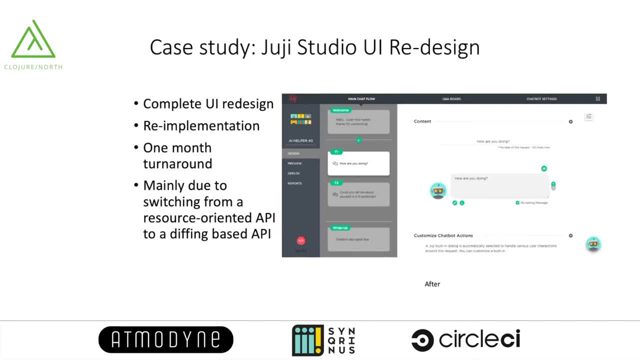 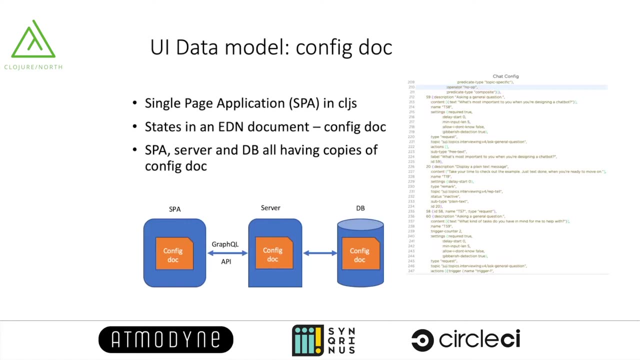 attribute the success meaning to our switching from my user usual resource oriented API to a different based API. so let's look at some details. 2g studio is a single-page application written in reframed. the UI states are all in an add-on document, what we call a config doc. it is basically a listed clear map. 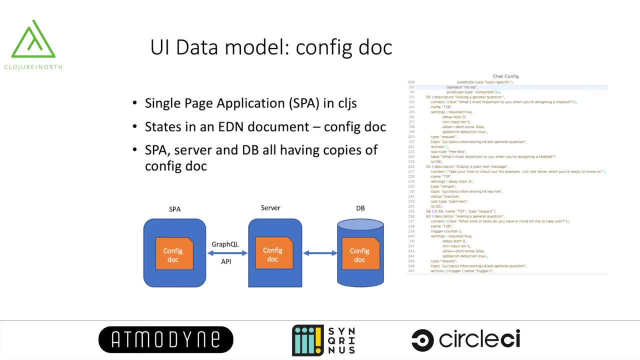 containing all kinds of information about, as a chat, configuration sections, topics, questions, follow-up questions, conditions and so on so forth. most of these have direct mapping to some UI elements on screen, so on the server side the same config doc is maintained. in addition, the config doc is persisted in the database, saved as a JSON document in postgres. so when 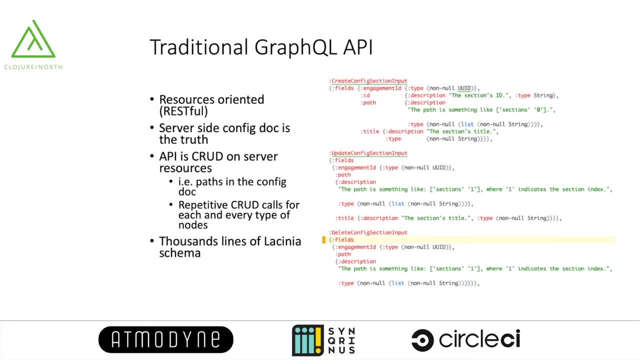 we started to develop 2g studio, we took the usual traditional approach, which is to treat the server-side config doc as a truth, because this is what being persisted in the database. so each path or each load of the config doc is a remote resources need to be managed in a REST formatter. also, we are using GraphQL for API, but 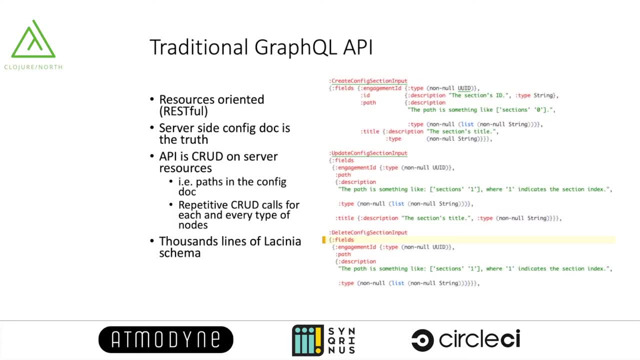 the model of client-server communication is the same as REST. basically web client conduct CRUD operations on remote resources on the server. to do that we have to write a lot of repetitive CRUD. GraphQL calls like this for each and every type of loads in our config doc. because I have many different types of loads of GraphQL schema file grows to be. 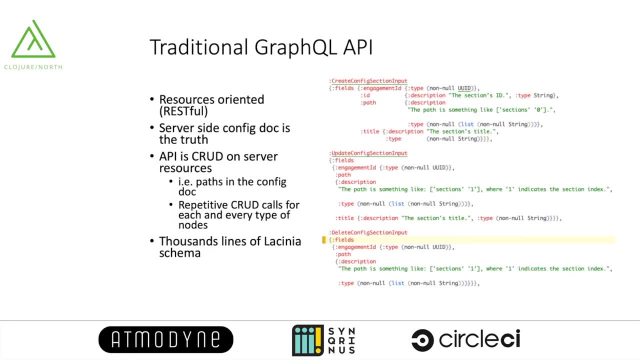 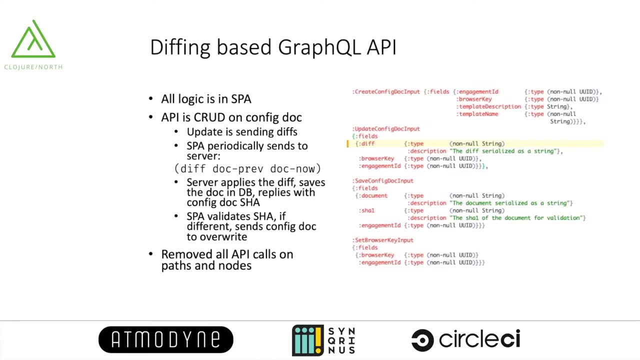 thousands of lines of add-on code, so I'll look at our new schema after we write. we now only do CRUD operation on the config doc as a whole. update the config doc becomes just sending the diff of the config doc. now all the logic is concentrated in the single-page application. 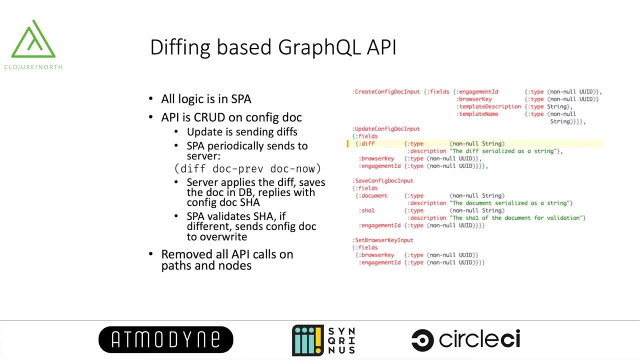 on the client side. the client periodically send these config doc changes to the server. the servernarly applies a diff to patch its own copy of the config doc, save the doc in the database and return a document char to the single-page application. so the single-page application validates. 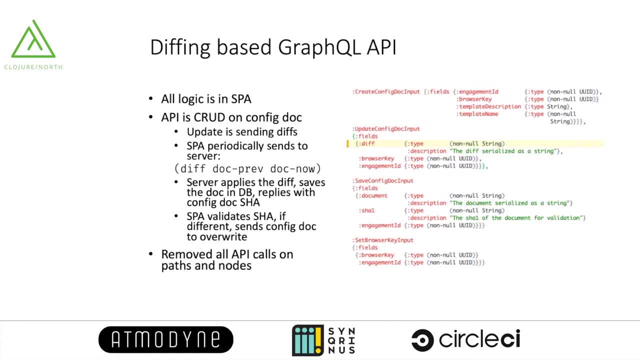 that the resultsarves of the 지� place received documentation. char is the same as its own char. and then consider its stack for big arrivingначs application is the same as its own char. and then马 SMB2s Buni this operation successful and continue its business. so all the api calls on different. 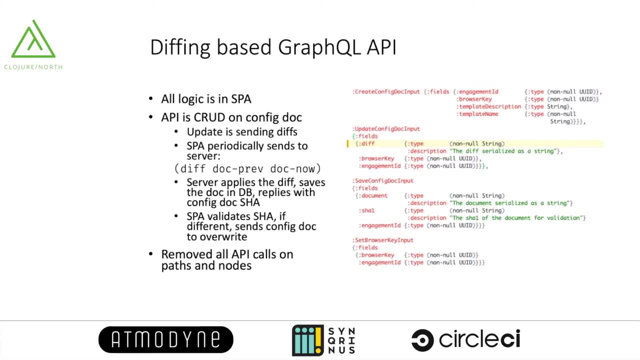 loads in the config doc are removed, replaced by a few api calls on config doc, create doc, fetch doc, update doc and save doc, which is front-end developers no longer touches once it was written, because the front-end developers has complete control of the data model and did not need to. 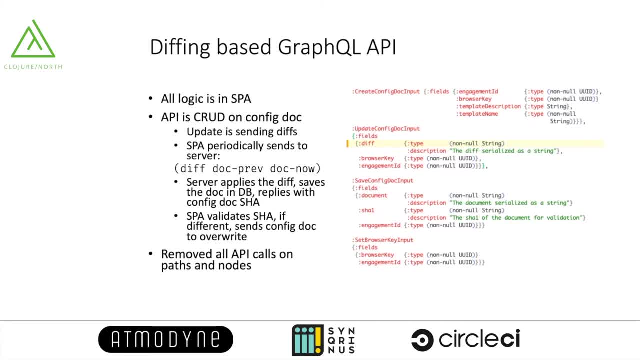 be concerned with the server side. they could quickly revamp the entire ui of juji studio. it took less than a month to go from design inception to the end of implementation. so the stiffing based api architecture is well suited to single page application, where the logics concentrated in the ui and the server side doesn't need to know what exactly the 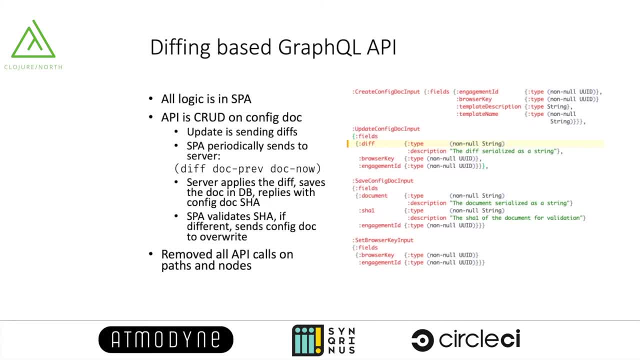 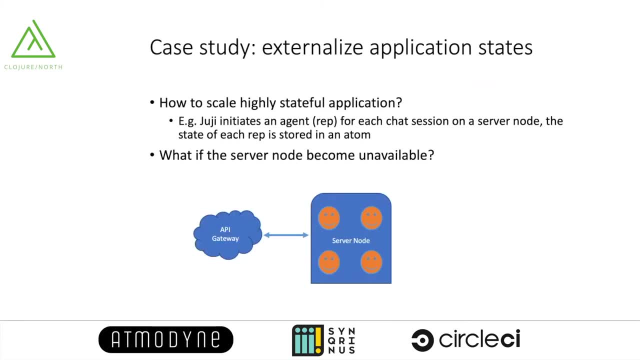 sba did. all it does is persistently move back to the default state. another use of diffing is to externalize application states so it is easier to scale, scale stateful applications. for example, juji creates a chat agent for each chat session. we call each such agent a rep. it's a shorthand for responsible, empathetic persona. 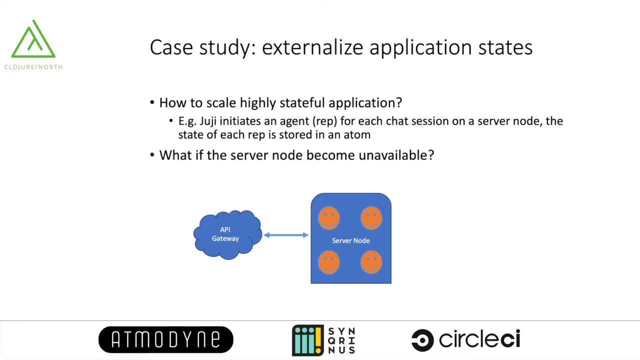 state, so to speak, which is stored in autumn, so each application server loads may contain many such running reps. when people, multiple people, can conversation, making conversation, our platform. so what if a server load goes down, become unavailable? we do not want to stop ongoing chat sessions, so one way to 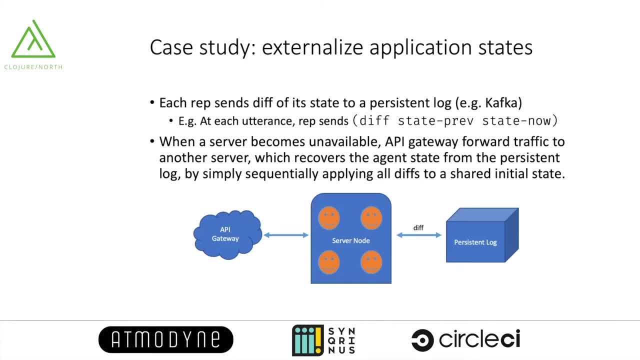 solve this problem is to externalize each reps state by also closely send gifts of its states to a processing log, such as a Kafka topic. so after each utterance a rep will save the teeth between its current state to its previous one. so this is a cheap operation and take a lot of storage when 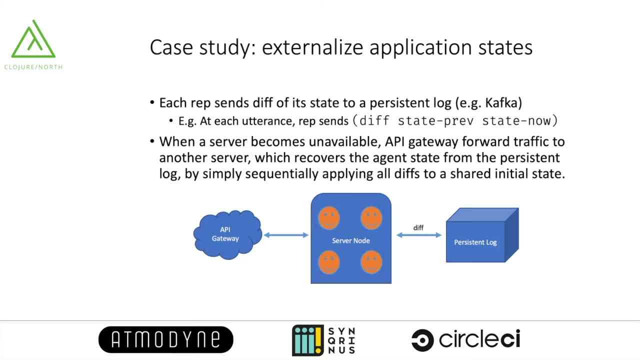 our server load becomes unavailable, the API gateway would forward traffic to another server load once a new server come up. it doesn't say the needed state to continue a conversation. it will fetch the teeth of the rep state from the persistent log and simply sequentially applying all the gifts to 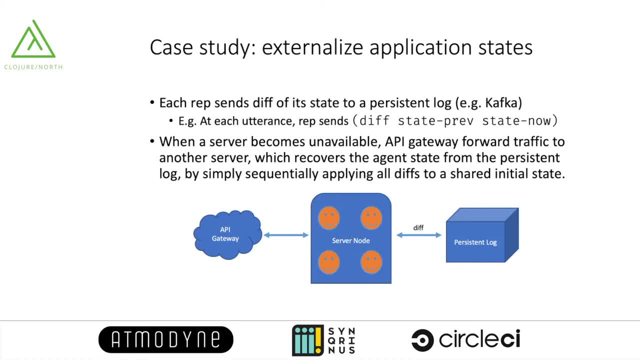 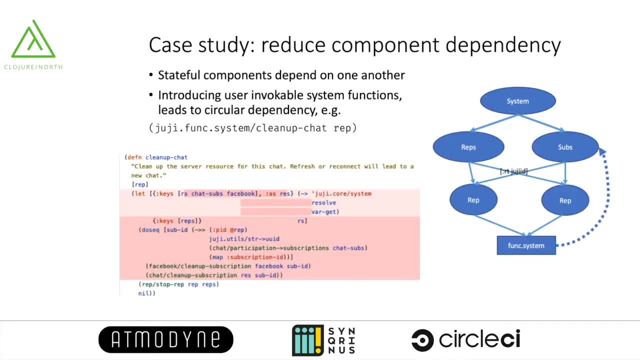 a shared initial state. so this will recover the rep state and then enable the conversation to resume. so far, we have only treated each teeth as a black box. the receiver of the teeth does not have to look at the content of the teeth. all you need to do is to. 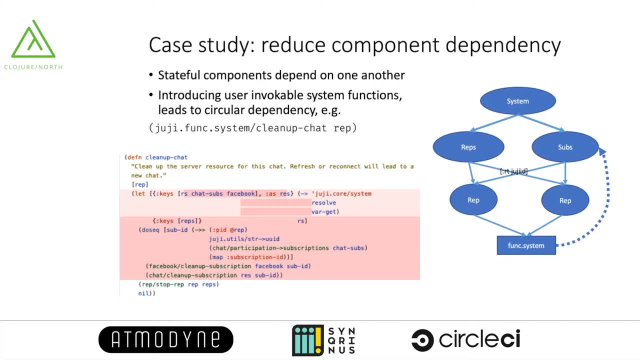 blindly apply the teeth. however, when it's necessary, teeth can also be inspected to extract the useful information. after all, a thief is just a piece of data. so here's an example. so we use two components systems to manage these stateful components. so one component, called reps, is a container for all the states of the reps. there are other. 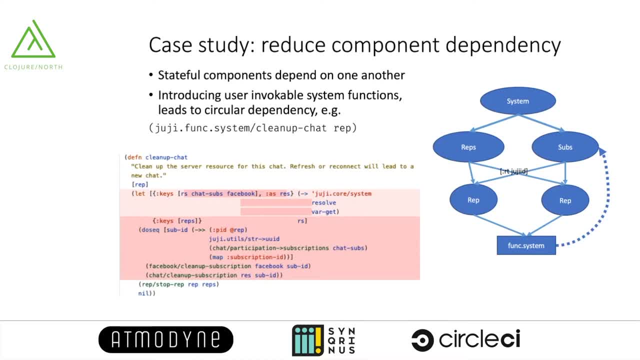 components that are containers for subscription data, such as there's a chart component for hoding web sockets gradually, our subscriptions and, or I think, channels for chat. there's a Facebook component for the data for both messages sharing and the hundred criteria. so each front page component has different. 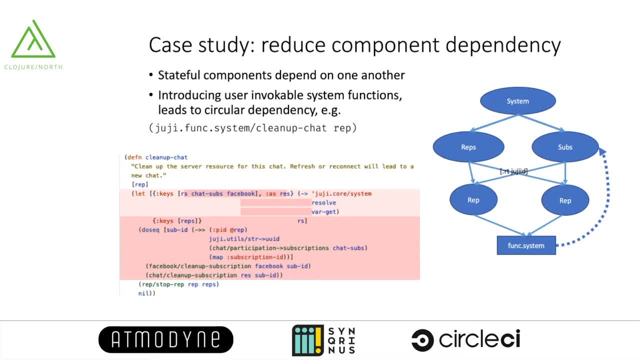 so these two components are shared and these bonus components share a number of contest for both recipes and gate into these X and alt quais to get my signals for holding pages and the page specific IDs and so on. So all those components live in their own namespaces. 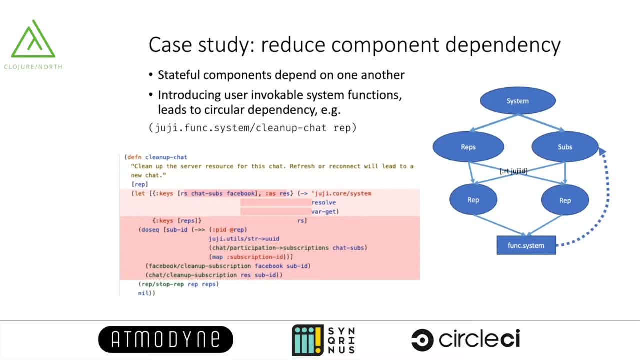 So when our chat is finished, this system resources needs to be freed or cleaned up. So since work well if all work is initiated by the system. However, since our chat support mixed initiative, the user may take initiative to terminate a chat, for example. 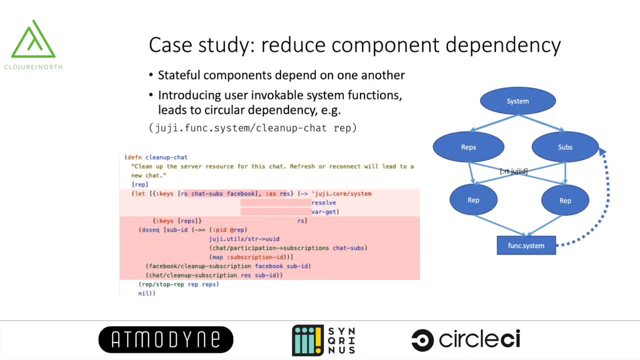 by saying goodbye or stop, and so on. A user level function now is needed to clean up the server resources, which requires access to the system level components. So such arrangement can easily get into a situation where you have circular dependency on your hand. For instance, here, Facebook and chat components contain some subscriptions. 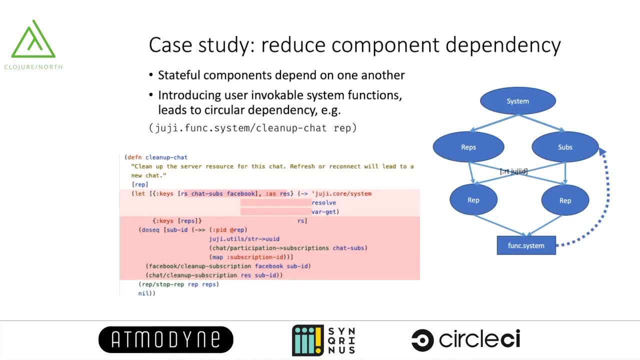 So, in order to free those subscriptions, a user level function- clean up, chat- have to depend on those components. But these components may also depend on, already depend on by the parents of those user level functions, creating a circular dependency. So, in general, 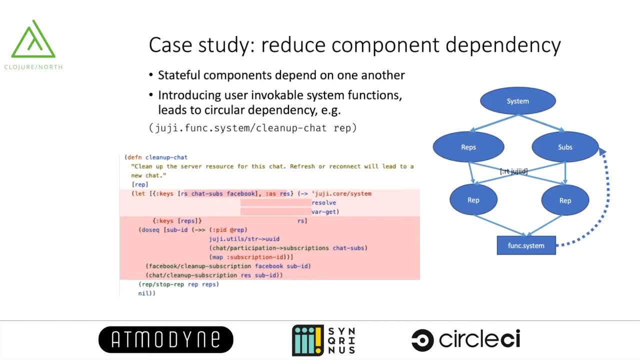 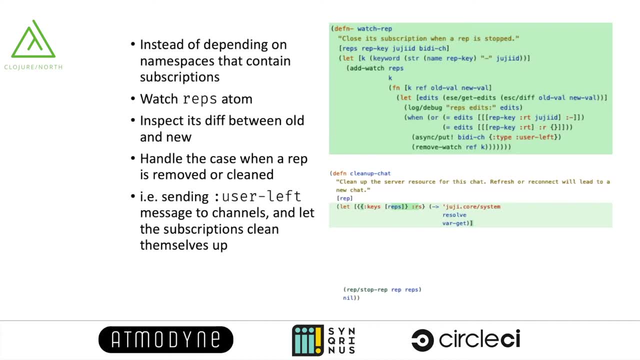 you will have a case of closed and coupled components To detangle those coupling. so in general, instead of depending on namespaces that contain those system subscriptions, our user level function can just watch the rep's autom. So when it changes we just inspect its diff between the old value and the new value. 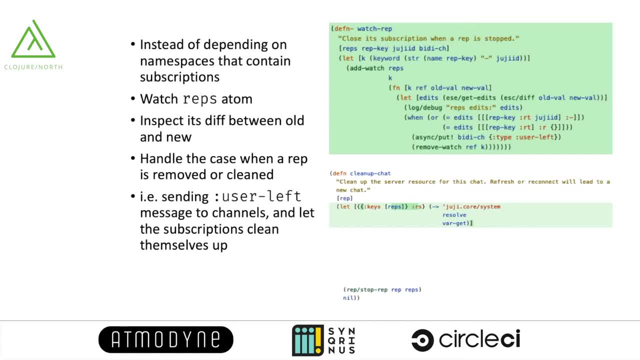 and try to match the cases where rep is removed or it's been cleaned. So once the desired match pattern is detected in the diff, the user level function can send the message to the chat channel saying okay, the user has left, which will automatically initiate the system level cleanup process. 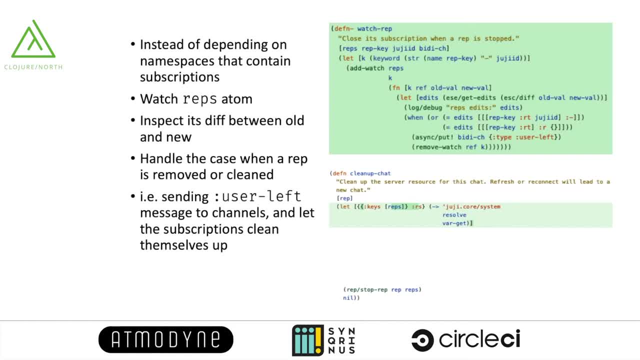 So this pattern of watching an autom that contains the value of another component, then perform different actions based on the content of the diff between the old and the new value. It's a very general way to detangle the dependency between components. So now hard-coded dependencies have been replaced. 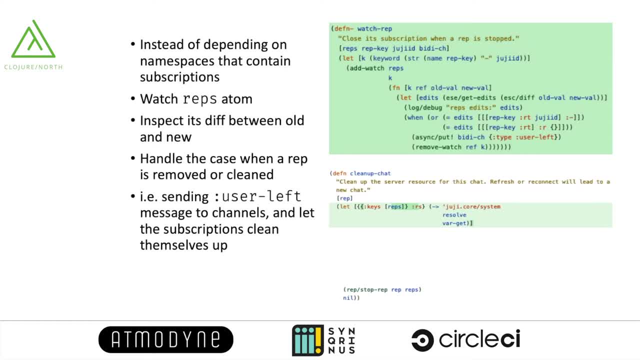 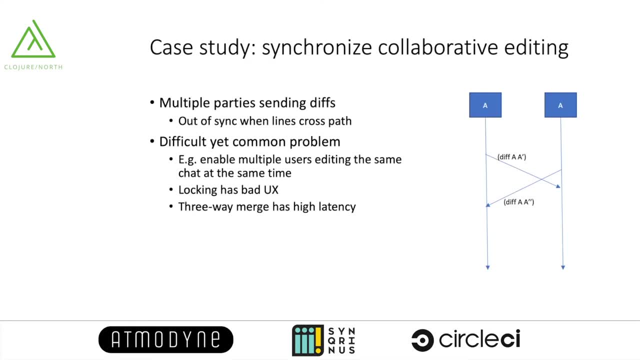 by flexible pattern matches. on diff data, So far we have only covered cases where one party sends changes to another party in the form of a diff. So what happens when multiple parties send diffs to the same data model at the same time? That's a difficult problem. 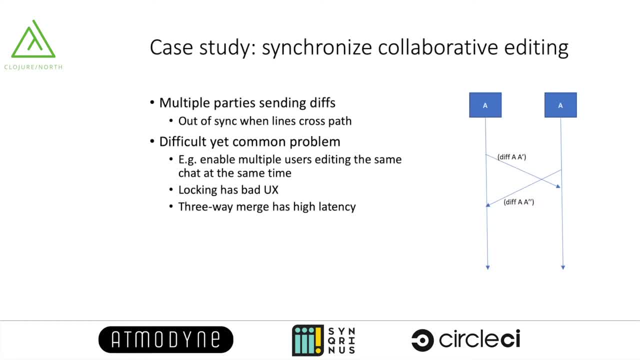 of collaborative editing. So in this diagram you have two parties sending diffs to each other, So when those lines cross, data can get out of sync because diffs may be applied on the wrong data. So this is a difficult yet common problem. For example, 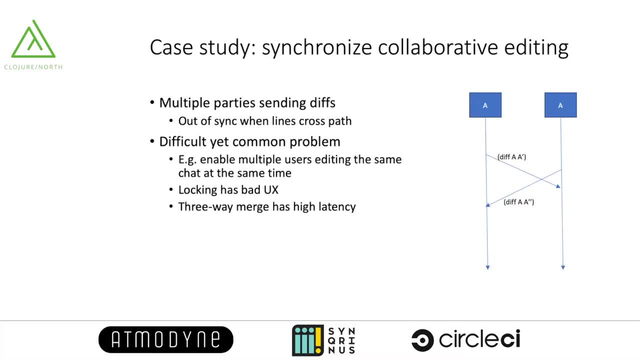 how to enable multiple users to edit the same chat. How to enable multiple users to edit the same chat at the same time in the GeoG platform. The traditional solution to this kind of problem includes knocking, which will forcefully serialize the updates so that there are no crossing lines. 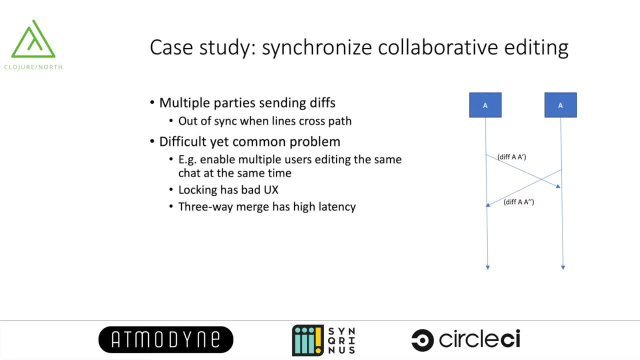 But the user experience is very bad because users have to wait in turns to edit the document. Another approach is for a selected cost to perform three-way merges of everyone's existing updates so far. then send back to everyone the merged version Again. the latency is bad. 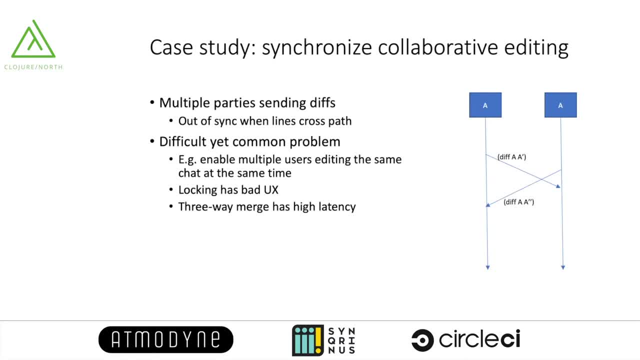 for this approach because updates have to be waited, have to wait for the end of the round trip of the three-way merges, So a single slow load will slow down everybody else. So it turns out there's another approach which is based on diffing. 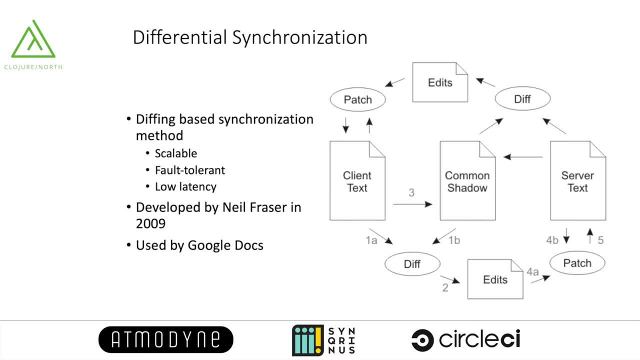 offers a better solution. So this diffing-based solution is called differential synchronization. It is a scalable, thought-tolerant and low-latency method for collaborative editing. It was developed in 2009 and it is what Google Docs use for collaborative editing. 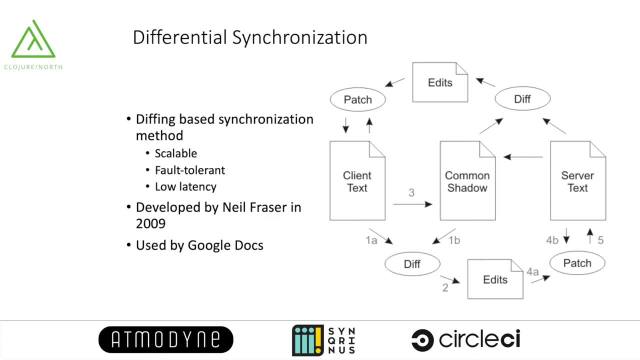 So let's take a look To simplify. first, let's assume everything happens on the same host. So in addition to the client and the server copy of the data, there's a common copy. It's called common shadow. So the client. 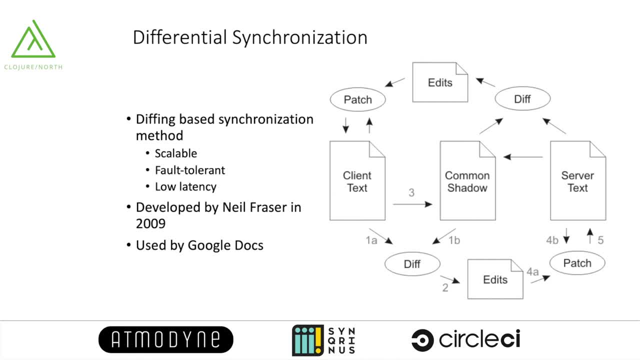 after done some editing, first computes a diff of its own data with that of the shadow, then saves its data in the shadow and finally sends the diff to the server. So the server takes the diff, applies the diff on its own copy. 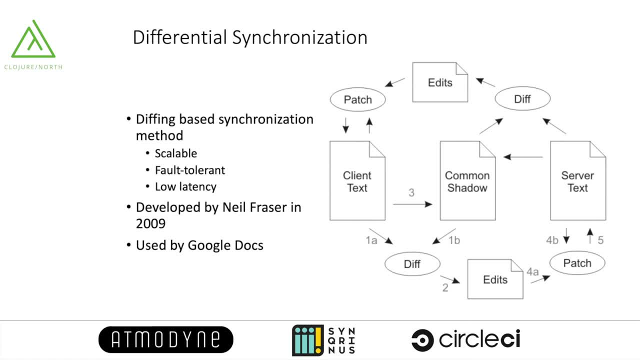 Now it repeats the same steps. in reverse, The server will do the diff between its own data and the shadow and then sends the diff to the client. So it's repeating the cycle, so the data becomes eventually in sync. So now let's look at 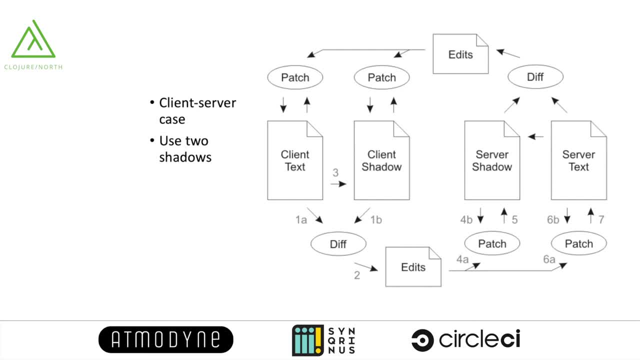 the realistic cases of the client and server live on different hosts, So we'll split the common shadow into a client shadow and a server shadow. So the rest of the algorithm is the same. The only addition is a char or checksum of the client's shadow. 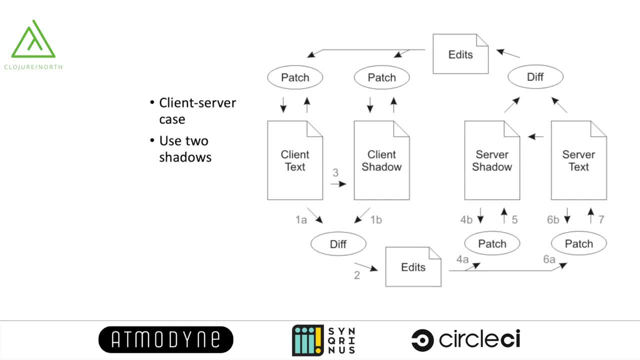 needs to be sent along with the diff, So the server shadow can be validated to be the same as the client shadow. So if the shadows fail to match, we'll send the whole document over to overwrite the server's copy. So like what we did. 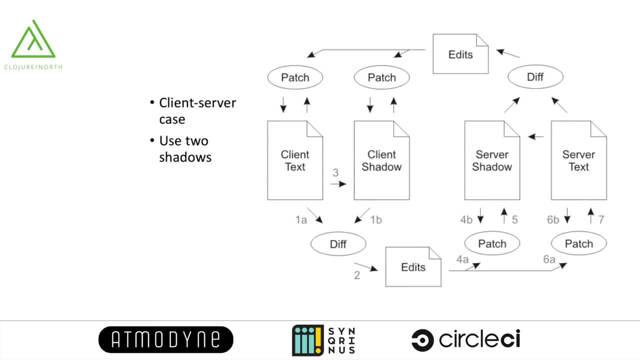 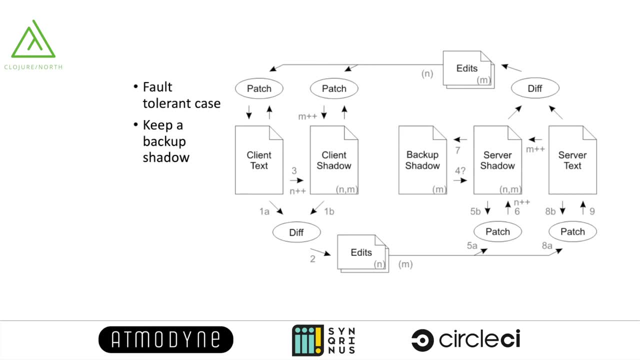 in our diff-based GraphQL API. So in the case of network outage or partition, data obviously will be out of sync for a while. Once network is restored, in order to resume synchronization, an extra backup shadow is needed on the server side To keep a previous state. 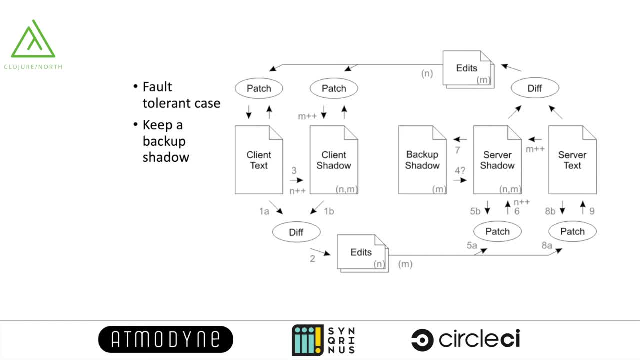 of the data. In addition, each copy of transmitted edits needs to be acknowledged, So a receipt should be sent when a batch of edits are received. So in order to do that, we also need a unique identifier for each batch of edits. So on acknowledged edits. 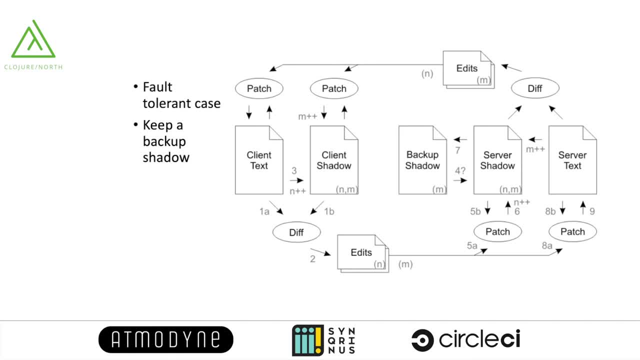 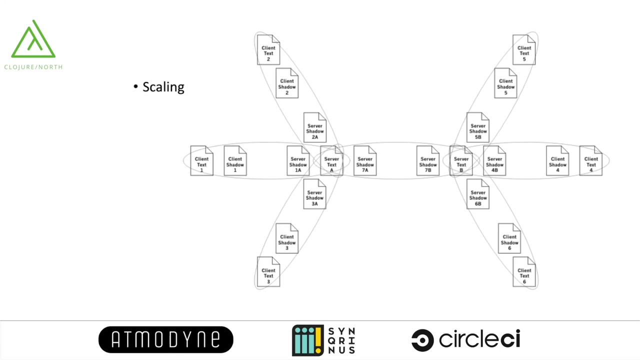 we'll be putting a queue. So when network is restored, the backup shadow will be loaded and the queued edits on the client will be sent over and applied on this backup shadow And then from there on the normal synchronization process will continue. So when there are more than two parties, 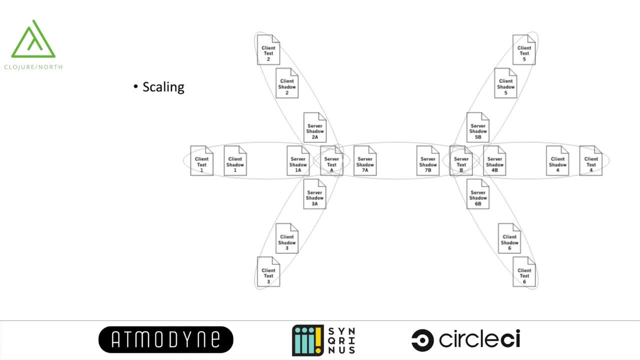 involved in the synchronization. some different topologies can be designed to duplicate a similar setup between a pair of hosts. For example, in this depicted topology, two server hosts synchronize with each other, while each synchronize with multiple clients of its own. So many other possible topologies. 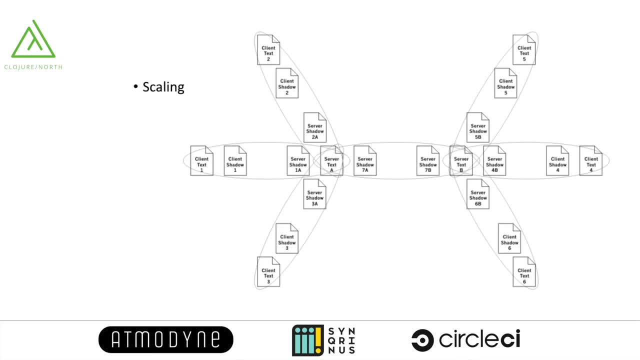 can be devised. So in general, this deep-in-based approach is scalable, fault-tolerant and performs well. The only limitation is that there can be only one edit transmission in-flight on the network at any given moment, But if the network speed. 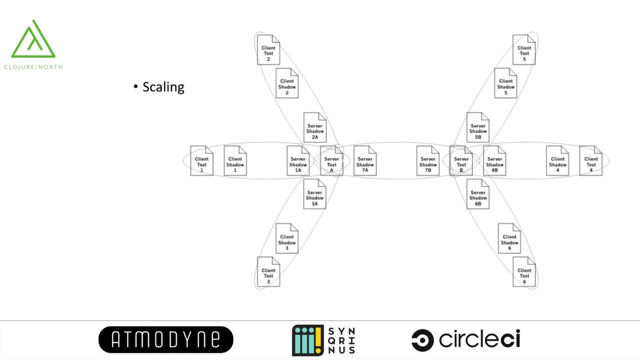 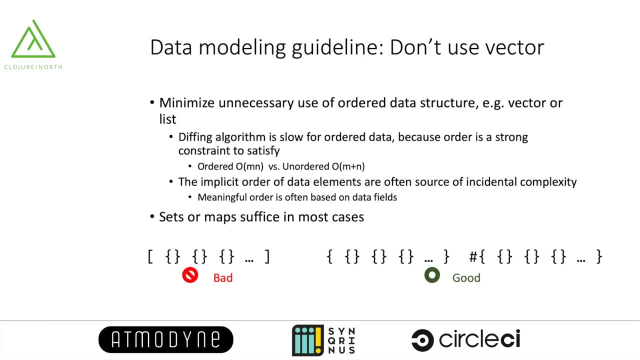 is acceptable, the user experience will be acceptable. So, before we conclude, we offer a recommendation for data modeling that is suitable for deep-in-based architecture. To dramatize our recommendation, our slogan will be: don't use vector, which actually means that. 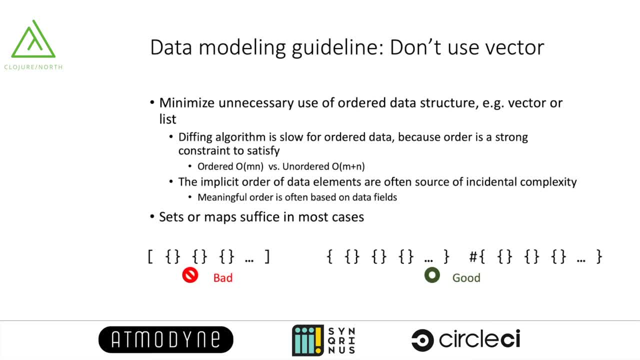 we need to minimize the use of ordered data structures such as vector or list. The reason is that deep-in algorithm is much slower for ordered data structure than for unordered data structure. For order, it is a very hard constraint to maintain, So deep-in algorithms. 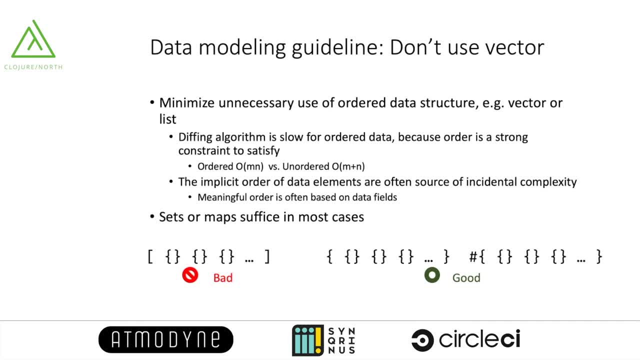 or ordered data is usually order of magnitude slower than unordered data, Where unordered data deep-in is just linear to the data size. for one pass to go through the ordered data is enough for deep-in them, But a transformation matrix is required for deep-in ordered data. 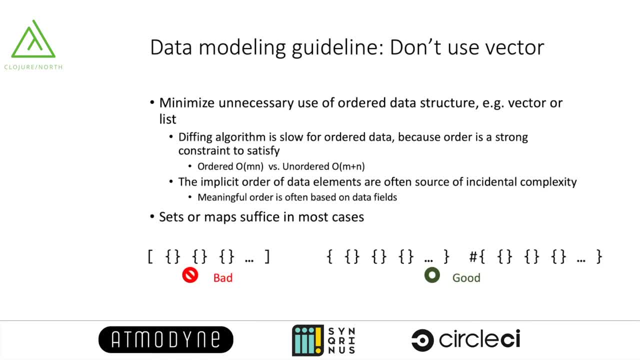 In addition, realistically, much of the implicit order we encounter in the real world are incidental, So we are likely introducing incidental complicity when we use vectors as a data model, because meaningful order is often imposed by the order in the data fields, not by the elements themselves.